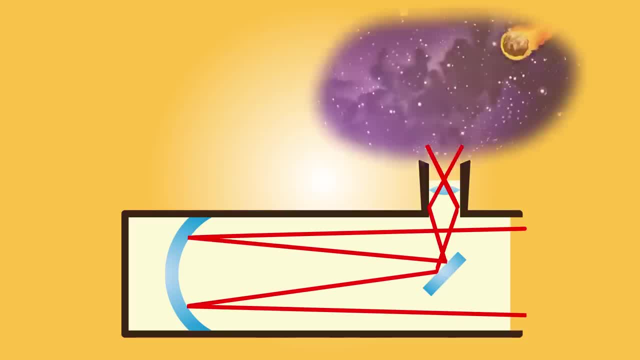 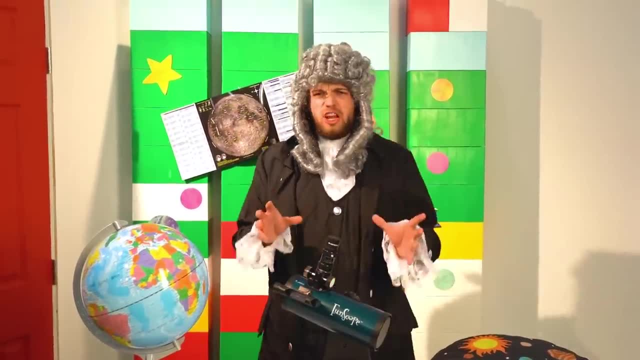 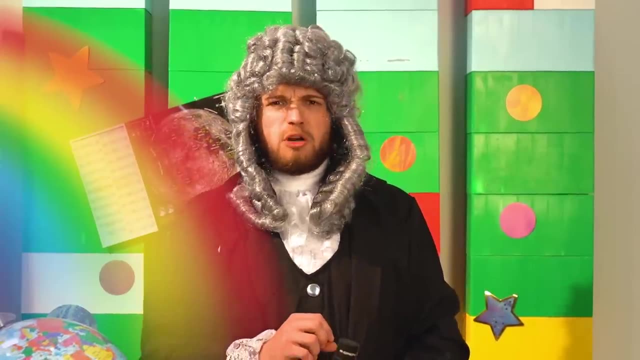 Isaac Newton discovered that curved mirrors reflect light. Curved mirror. Isaac Newton discovered that curved mirrors reflect light. mirrors can be used to improve telescopes. Yes, yes, I did. Those other telescopes would create a chromatic aberration. That means a rainbow effect. Is that what you kids are? 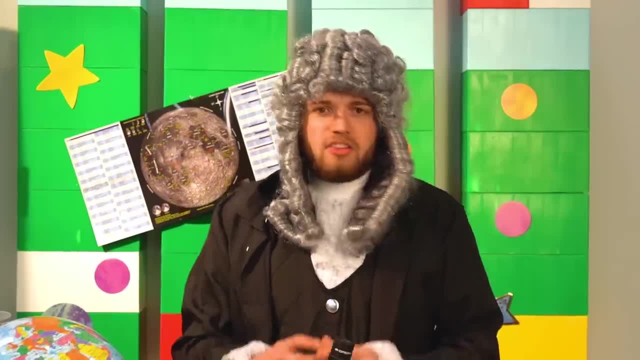 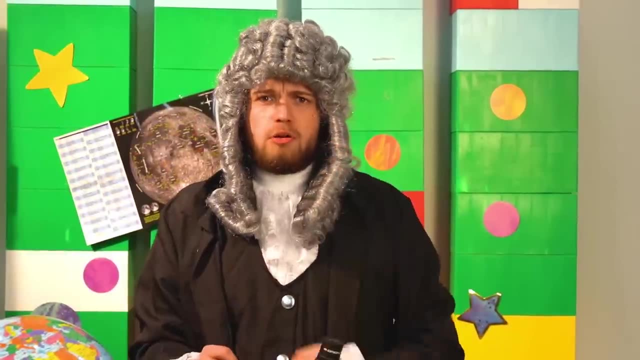 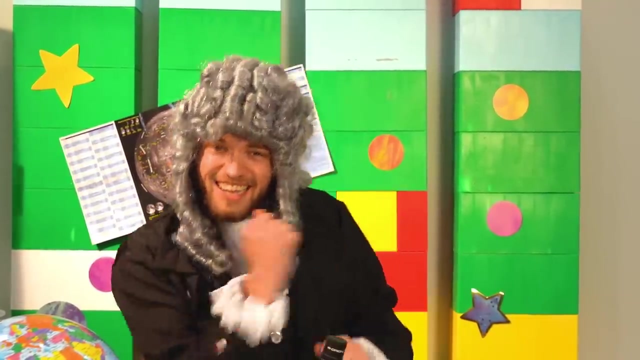 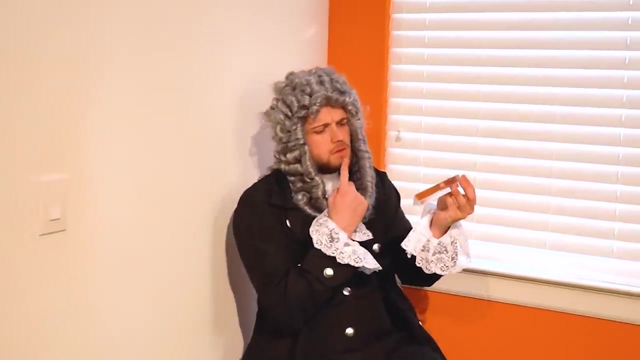 calling it now. Well, yes, These colors, these rainbows, they kept showing up and I had to solve the problem. And I did. But then I had to understand the problem. Isaac Newton's studies led him to figuring out lights and colors. One day he was sitting with the prism. 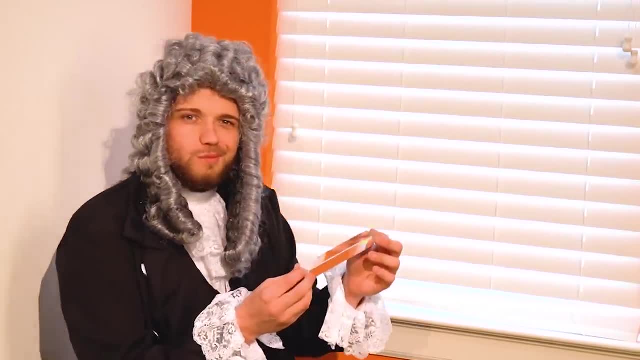 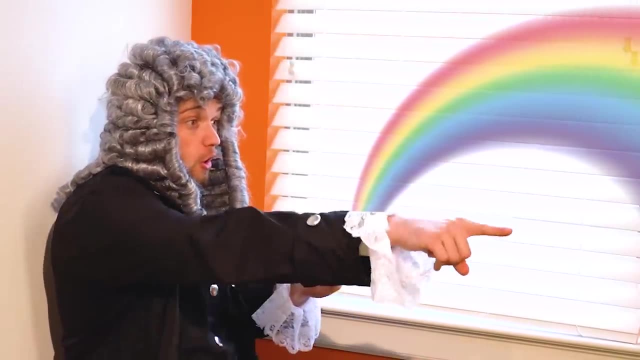 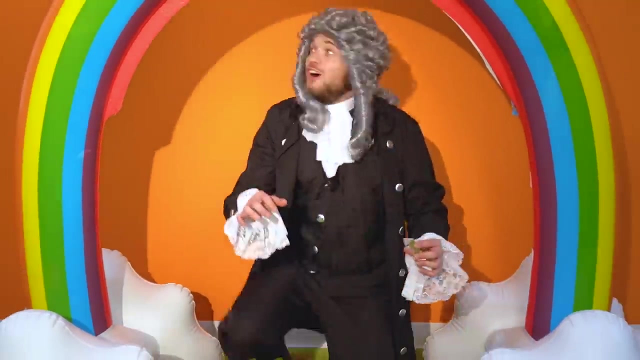 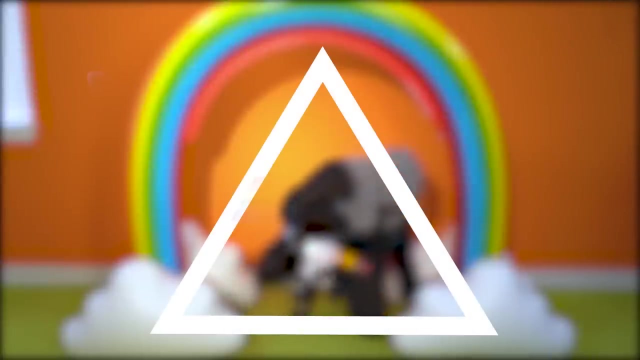 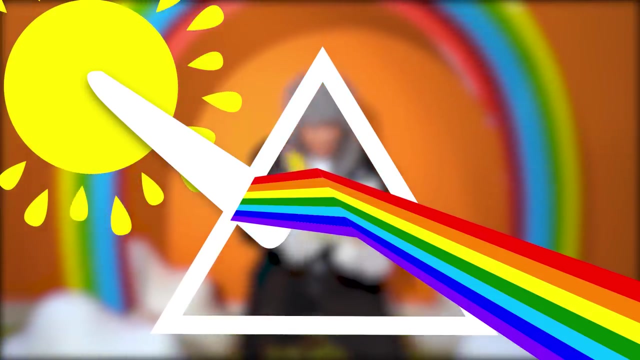 up to a window and then, I wonder, the prism projected a beautiful rainbow. Wow, all those wonders, Beautiful colors, Oh, magnificent. I've got to write this down. Isaac Newton was the first to understand that when you bend white light, the rainbow is revealed. Precisely I figured. 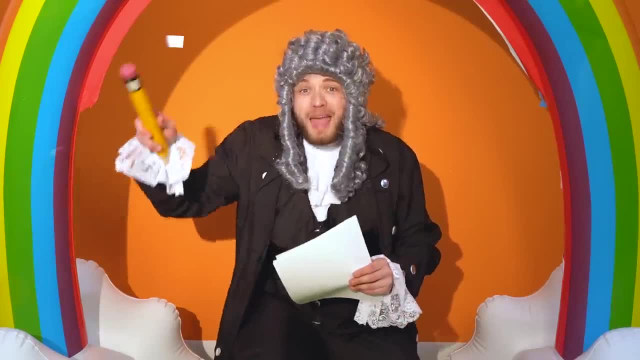 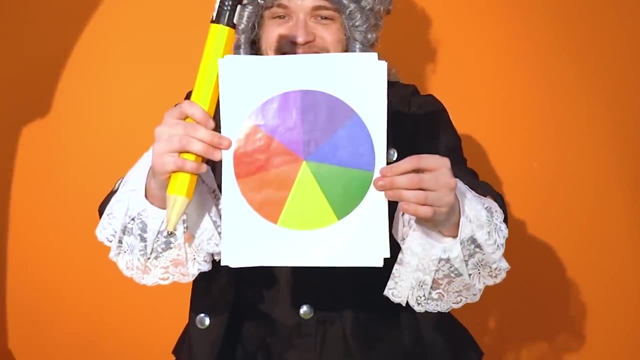 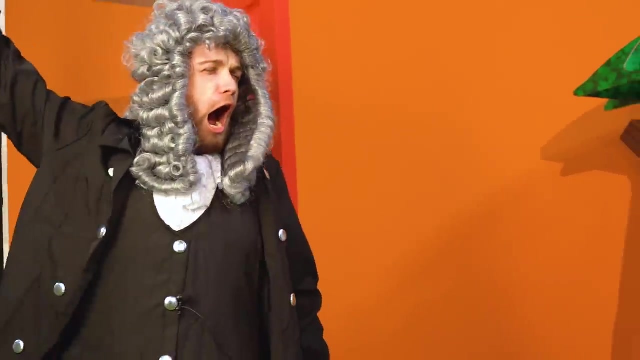 out that prisms don't color light. they bend white light to reveal the colors. The circle color wheel become the model for many color systems that we use today. Even after all of his research and discoveries, Isaac Newton wasn't finished yet. That's enough discoveries. 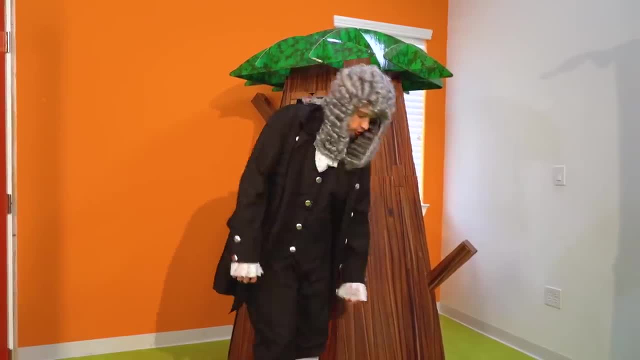 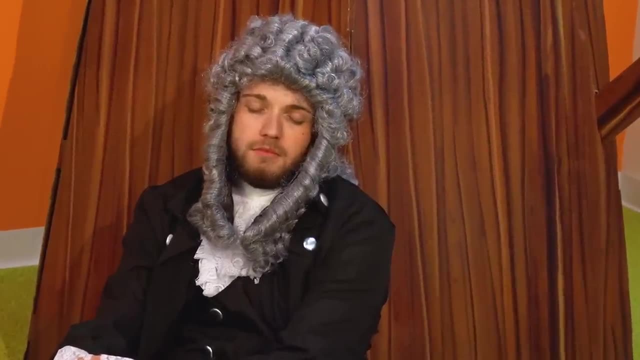 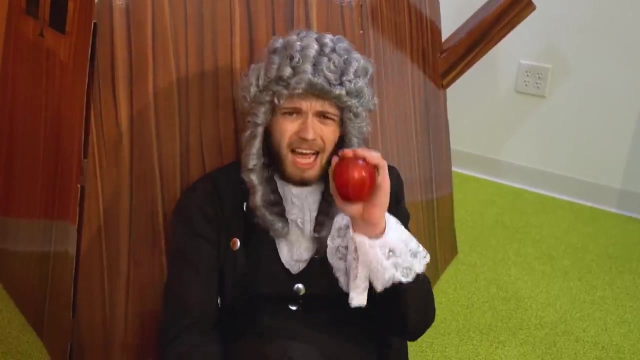 for now, I think I'm going to take a nice nap by this apple tree. One day, Isaac Newton was hanging out under an apple tree when an apple fell on his head. Huh, What, What was that An apple? Did someone just throw an apple at my head? 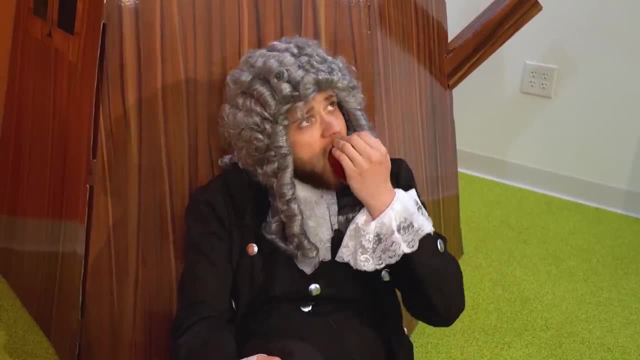 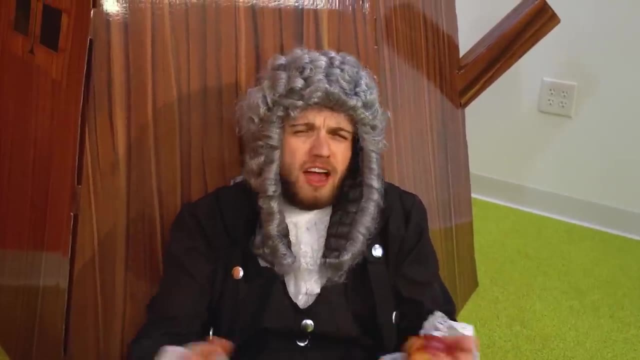 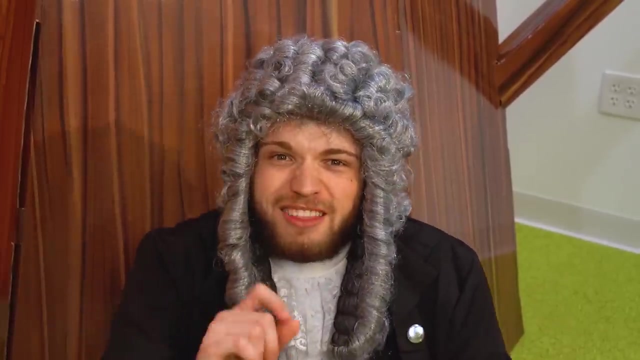 Isaac Newton was curious. He wondered why things fall down instead of falling up into the sky. Why do things fall down? Why doesn't everything just fall up instead of? oh? I think I feel another discovery coming on. Newton discovered a new discovery. 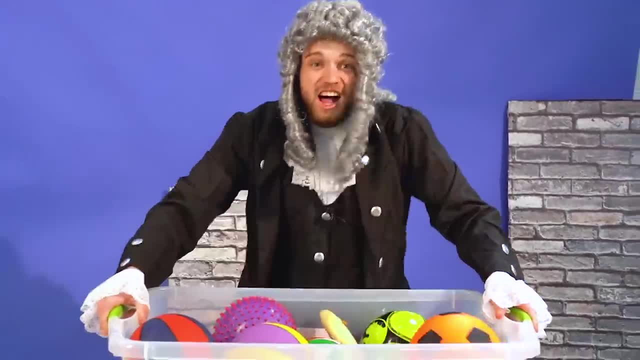 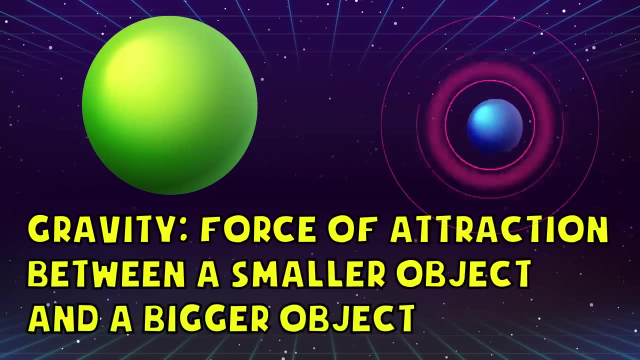 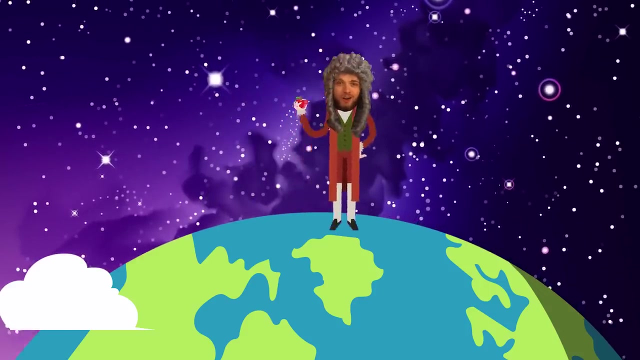 He discovered a force called gravity. I will call this gravity. Gravity is the force of attraction between a smaller object and a bigger object. The earth is our biggest object. This is why objects fall down. Oh, gravity, gravity, gravity, Wait. 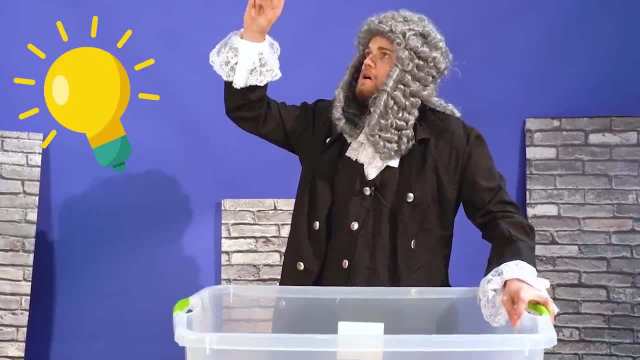 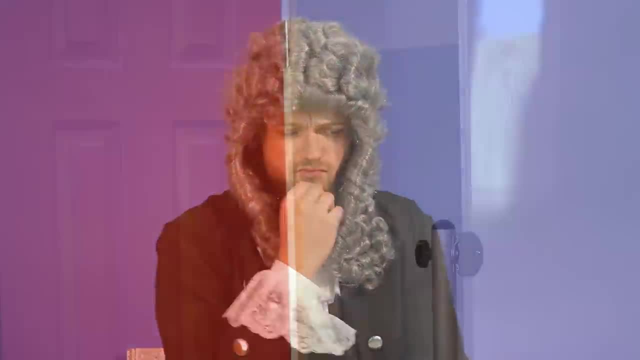 Isaac Newton was on the edge of another breakthrough. How does gravity fall down? How does gravity affect an object's motion? Good question, Hmm, Aha, I've done it. Isaac Newton came up with three laws of motion. Law number one: 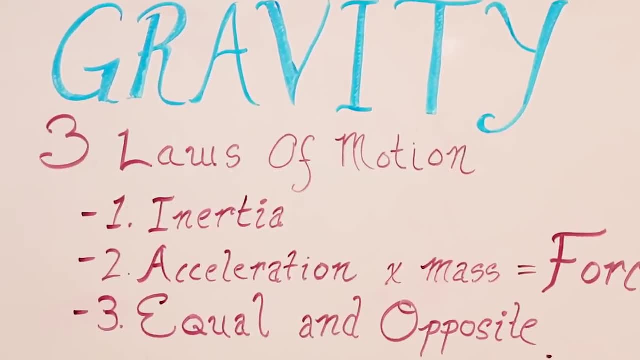 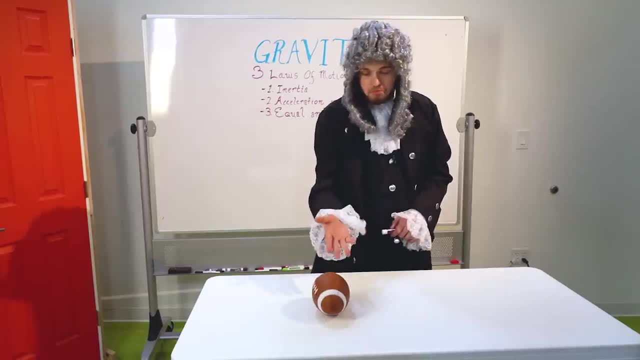 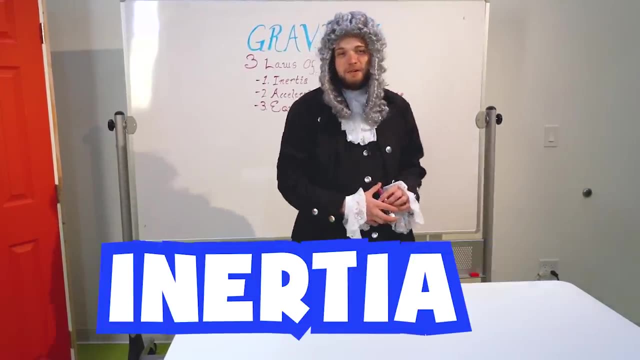 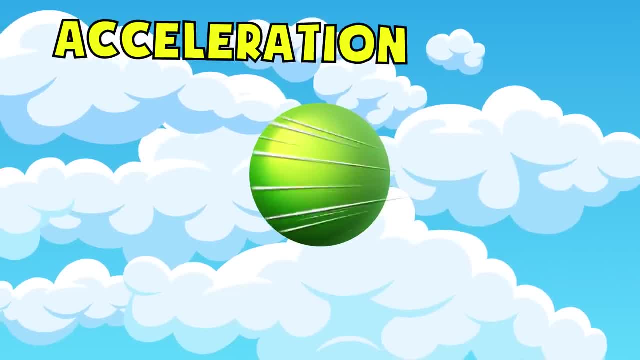 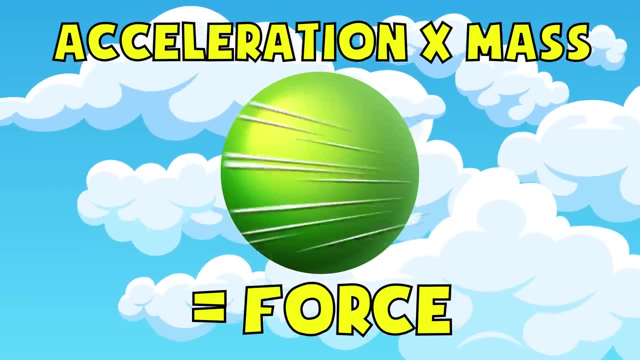 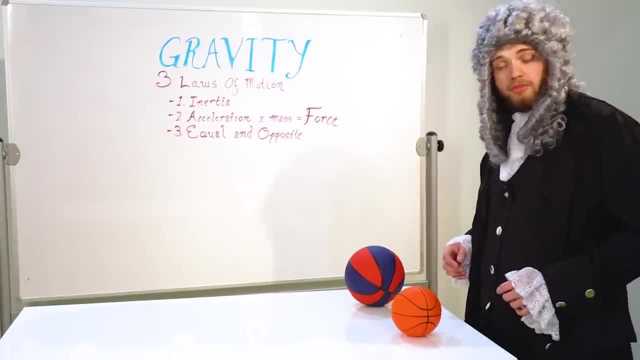 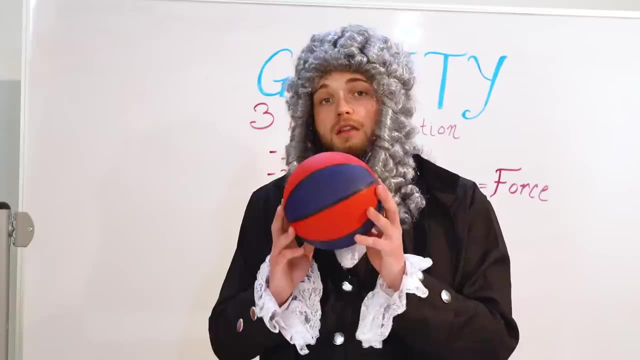 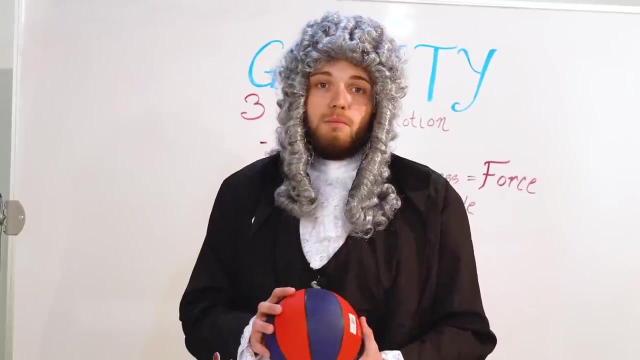 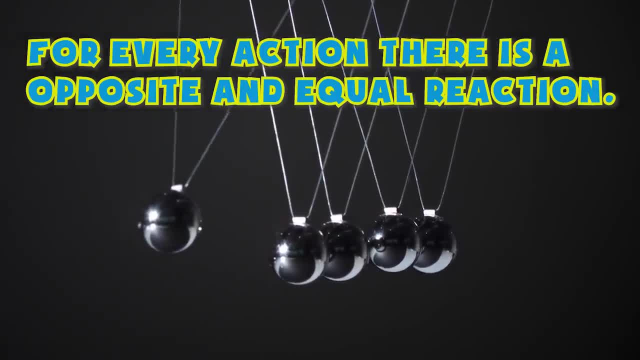 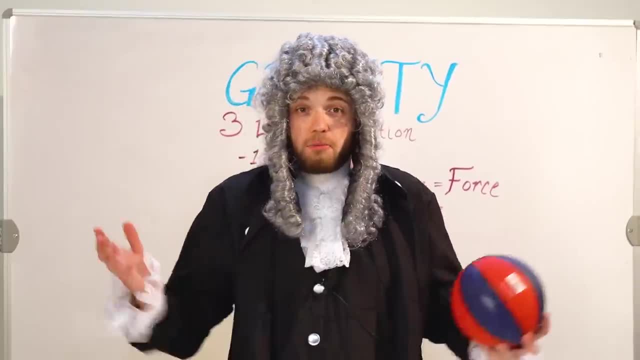 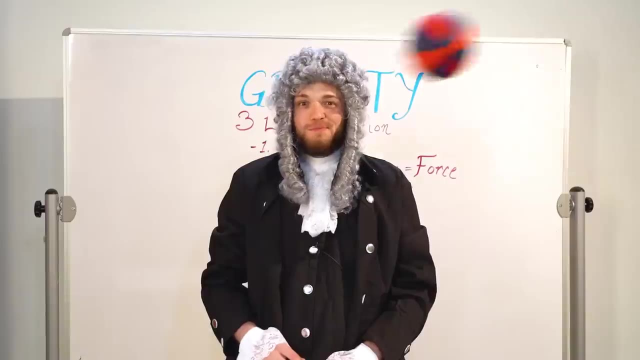 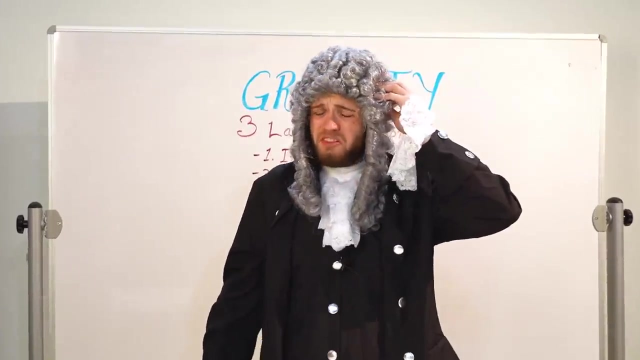 action there's an equal and opposite reaction. so if I throw this ball into the wall as hard as I can, it will stop it right. oh, I don't think that's a good idea. ah how the ball bounced back and hit me in the head with the same amount of. 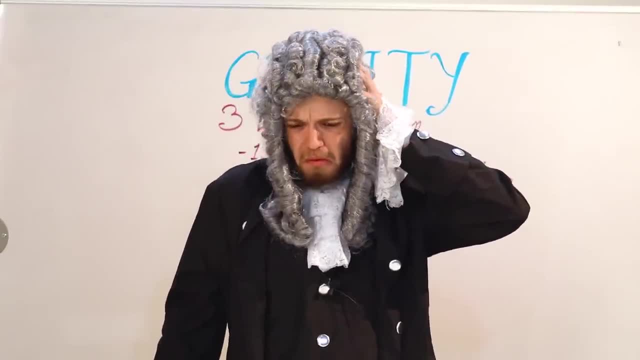 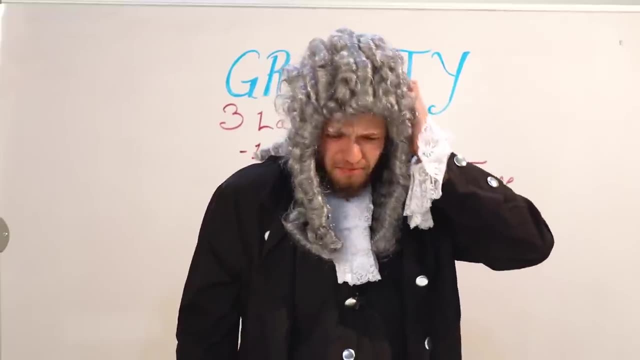 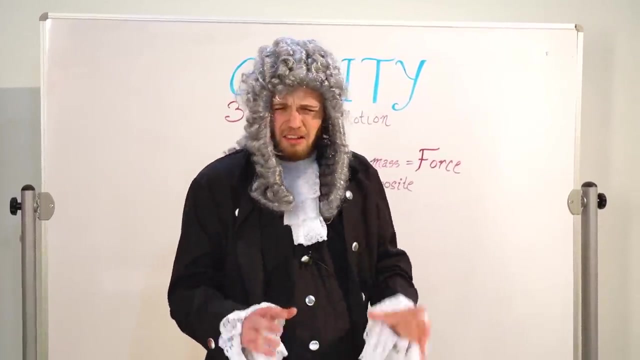 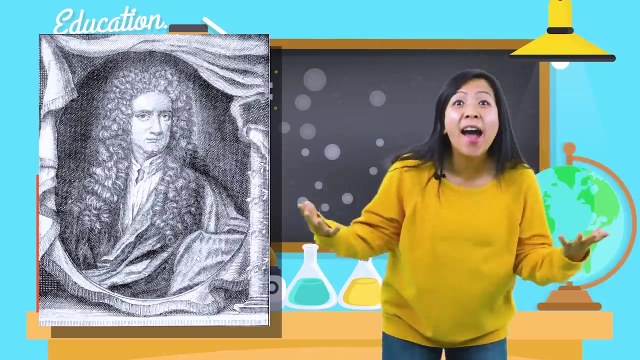 force that I threw it, so the ball hit you with an equal and opposite force. you used just like when you threw it at the wall. yes, so you understand to all of my laws of motion. now, huh, I think that's all my discovering for now. you all take a quiz while I go ice my head. wow, Sir Isaac Newton became one of. 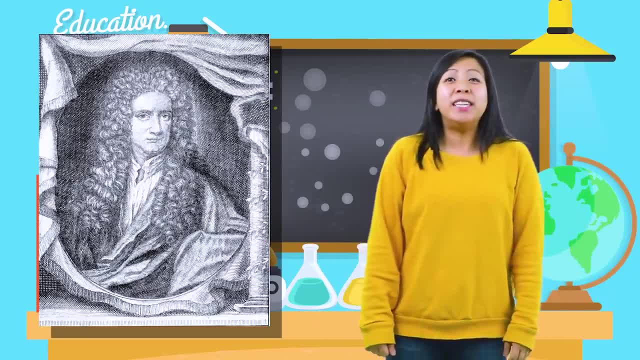 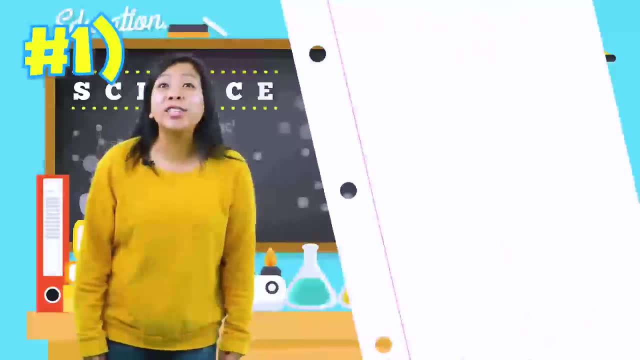 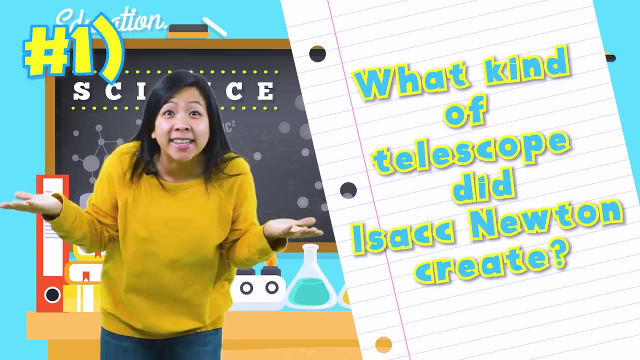 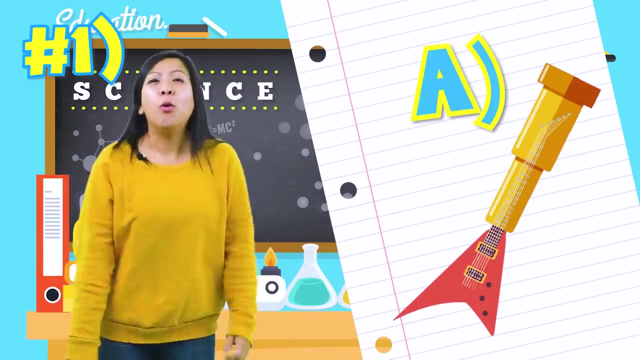 the most famous and influential mathematicians and scientists ever. Let's see if we can remember why. Question Number One: What kind of telescope did What did Sir Isaac Newton create? Is it A guitar telescope Or is it B pizza telescope? Yum, yum, yum, yum yum. 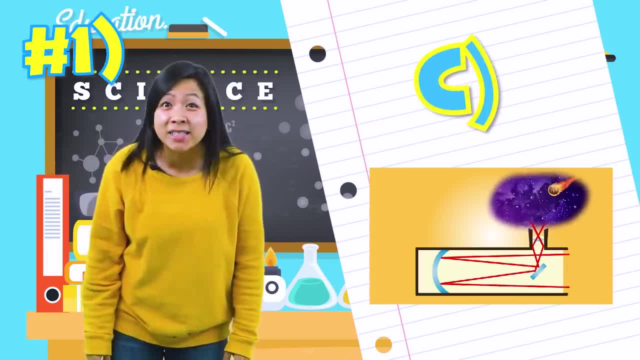 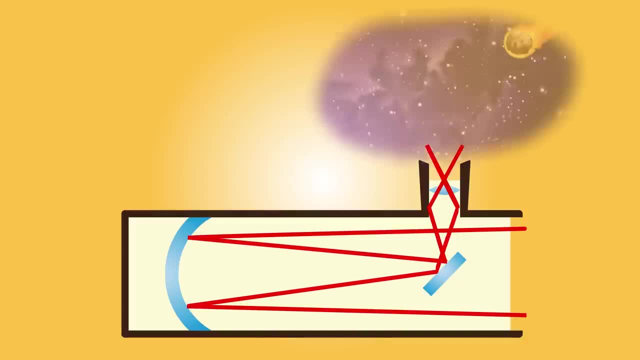 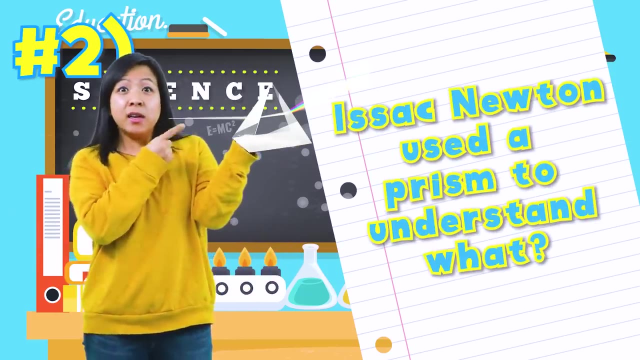 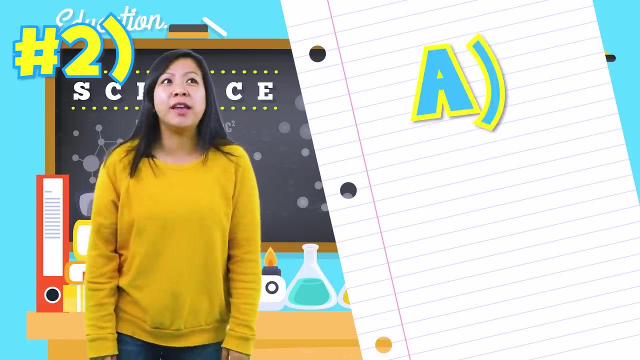 Or is it C reflecting telescope? Did you guess it? The answer is C reflecting telescope. Question number two: Sir Isaac Newton used a prism like this to understand what Is it A. he used a prism to understand the taste of French fries. 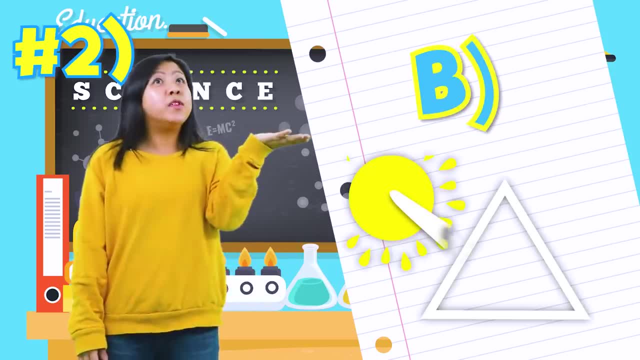 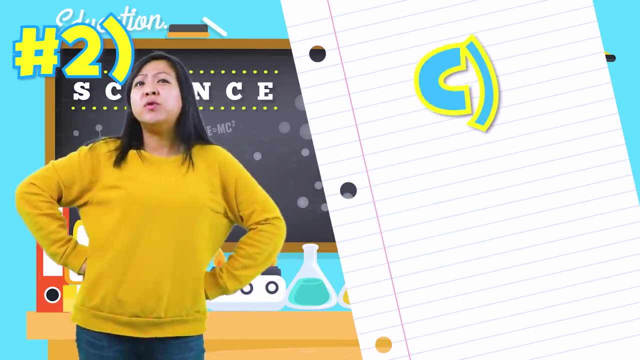 Or is it B? how white light refracts into colors of the rainbow. Or is it C? Sir Isaac Newton used a prism to understand the taste of French fries. Or is it A? he used a prism to understand different kinds of dinosaurs. 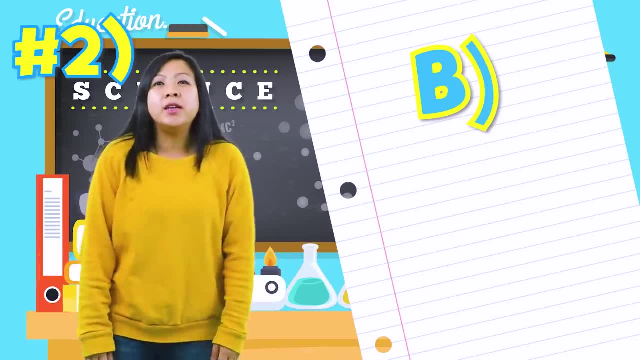 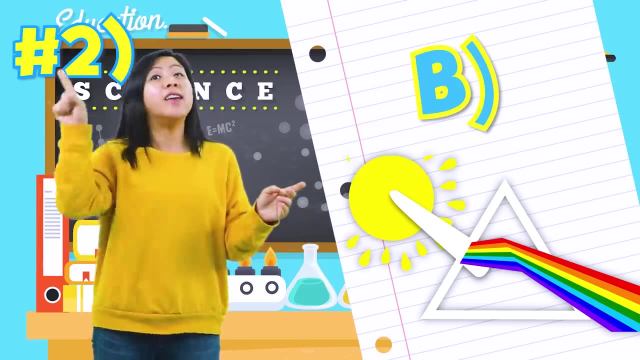 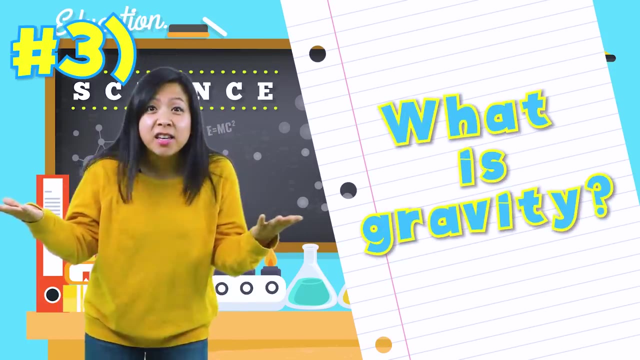 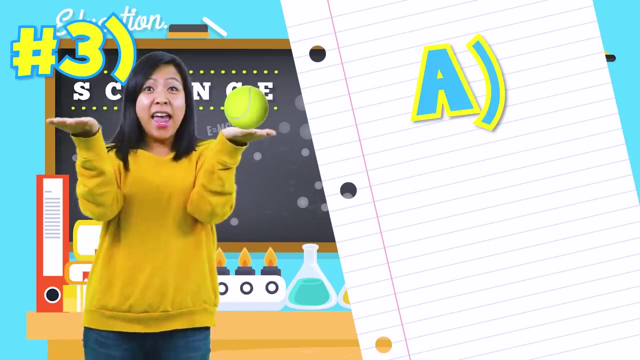 Did you get the answer right? It is C. Sir Isaac Newton used a prism to understand how white light refracts into colors of the rainbow. How cool is that. Question number three: What is gravity? Is it A a force of attraction between a small object? 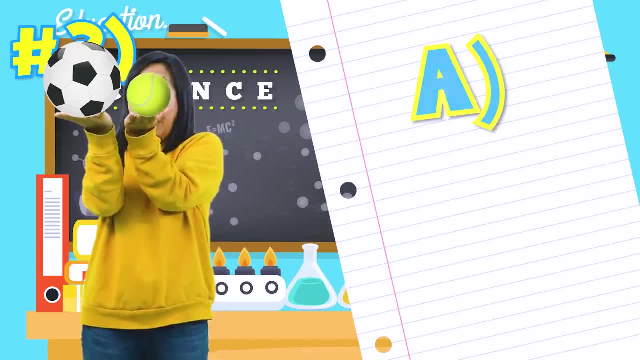 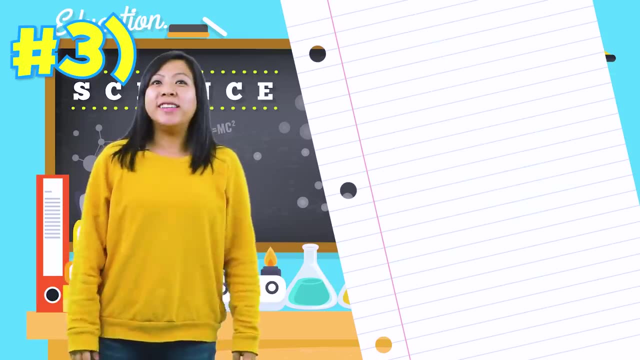 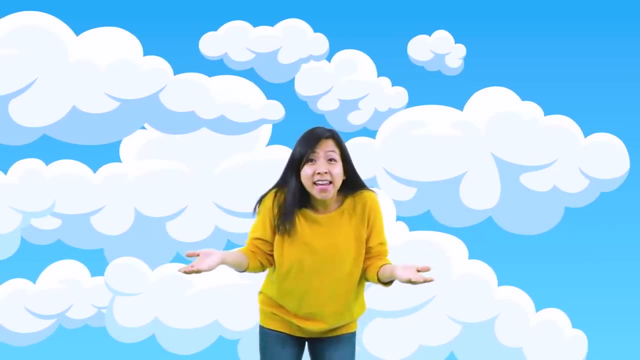 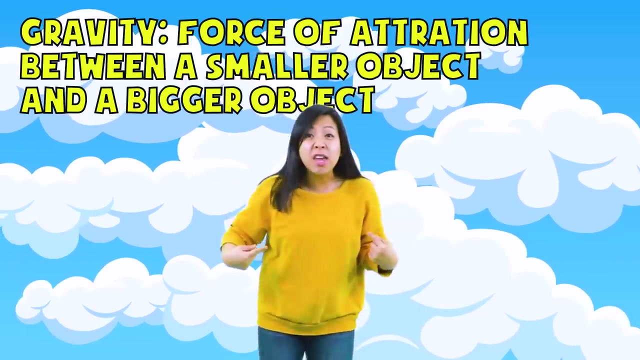 and a bigger object, Or is it B? is gravity a continent, Or is it C? is gravity a fish? Did you guys guess the answer? It is A. gravity is a force of attraction between a smaller object like me and a bigger object like the Earth I'm standing on.